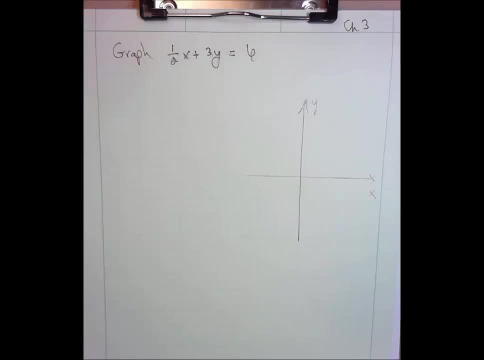 Let's practice a little bit with graphing a linear equation. This topic is found in chapter 3 of your Alex Integrated textbook. I'm sure all of you have vague memories of doing this in the past. Generally speaking, when we're trying to graph linear equations, a very popular thing to do is play the y equals mx plus b card. 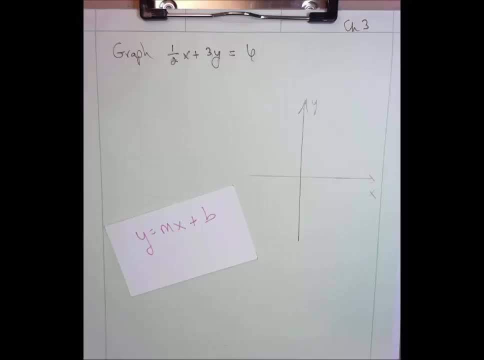 This is the most famous version of the equation of a line. Everybody probably remembers that if you can rearrange your equation into this form, the value of m is your slope and the value of b is your y-intercept. In this problem, we will play the y equals mx plus b card by rearranging our equation to get it to look like this: 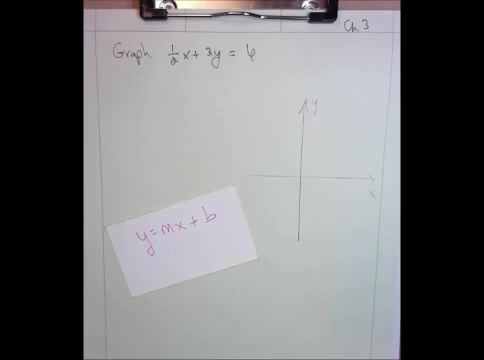 We'll pick out those values and draw using those. In the next example I'll show you a slightly different method of figuring out the positional- The positional of a line, which, frankly, I think is a little bit easier. But this is popular, so what the heck, we'll go with it. 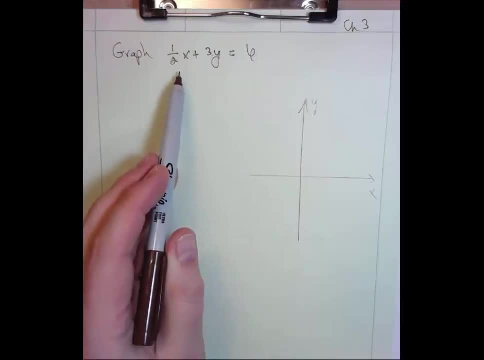 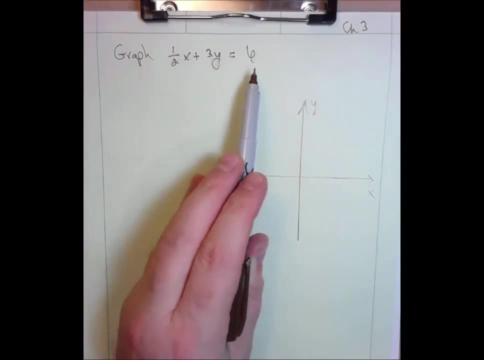 So I'm going to start manipulating my equation to leave the term with the y on the left-hand side and the term with the x moved over to the right-hand side. Just like with generic solutions to equations, I'm in charge of this expression. 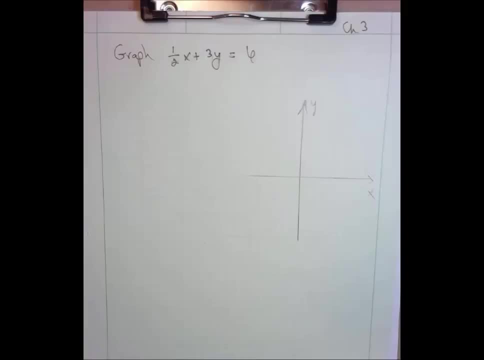 I am free to do anything I want to it, just about as long as I do it properly meaning I have to do the same thing. I am free to do anything I want to it, just about as long as I do it properly meaning I have to do the same thing. 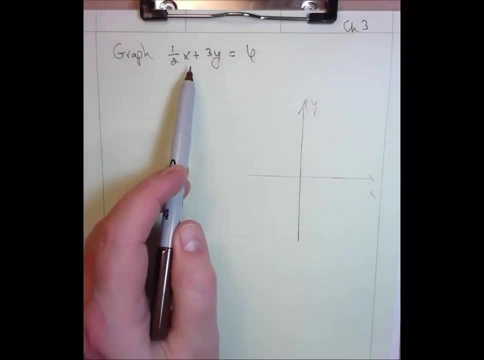 I would like to see this term with the x disappear from the left-hand side, and so I can subtract 1 half x from the left-hand side to make that happen. That means I also have to subtract a 1 half x on the right-hand side to maintain the equality. 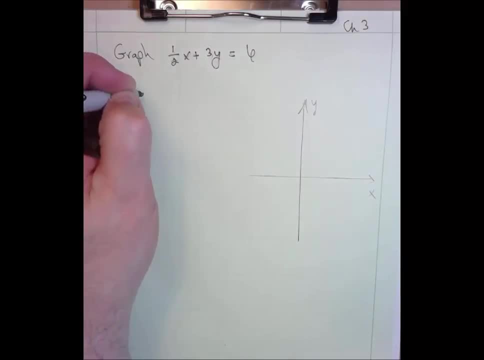 So I am in my head subtracting 1 half x from the left-hand side. That will leave the 3y alone on the left-hand side. This six is still sitting over there on the right, joined by now the minus 1 half x which is included on that right-hand side. 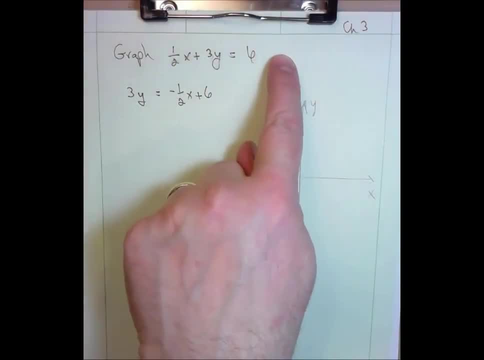 So it's just like we took this term just swoop, moved it over there by subtracting it from both sides. I put the subtraction of that term to the left of the 6, again, just because I'm keeping in mind. my y equals mx plus b card. 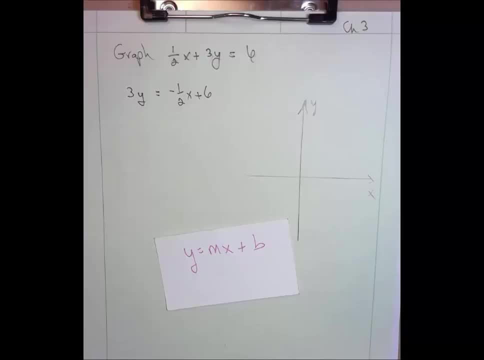 and I usually want the variable x term to the left of the constant. All righty. and now to isolate y, I want to divide both sides by 3.. So I'm just making a little note there that I'm about to divide by 3.. 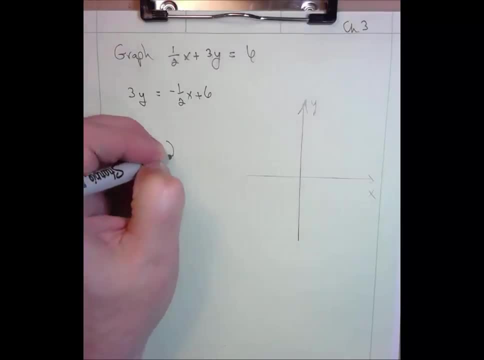 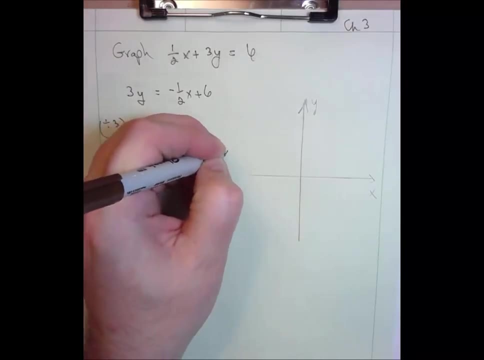 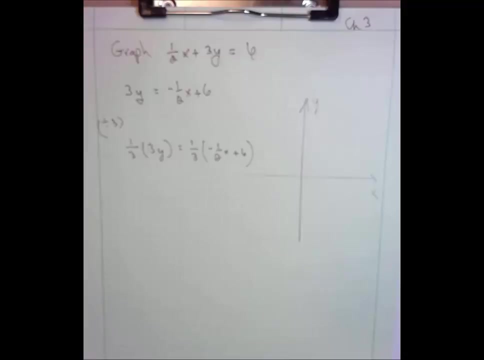 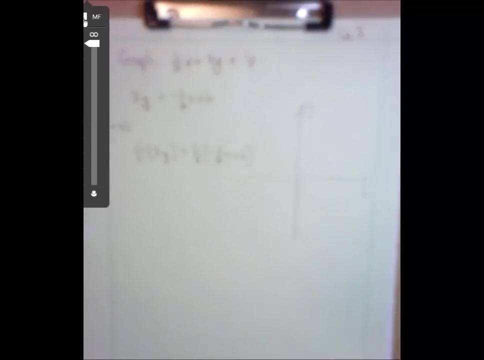 Or equivalently multiply by 1 third. and maybe that's a good idea here, because I'm going to be doing fractions of fractions there on the right-hand side, So maybe it's useful to see The division by 3 represented as a multiplication by 1 third. 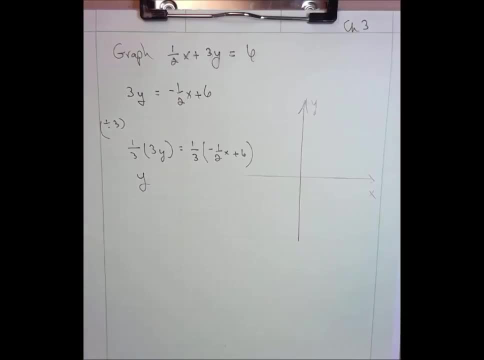 There we go, better focus. So I end up with a y on the left-hand side And then over here 1 third times negative. 1 half is negative. 1 sixth x, And then 1 third times plus 6,, 6 over 3, that's a 2.. 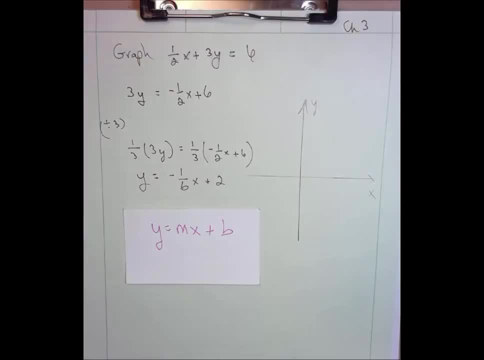 And so. So one more time, showing that y equals mx plus b card. I now see the slope and the y-intercept. for this particular item, for this particular line, I will have a slope of negative 1 sixth, which means my line is going downhill. 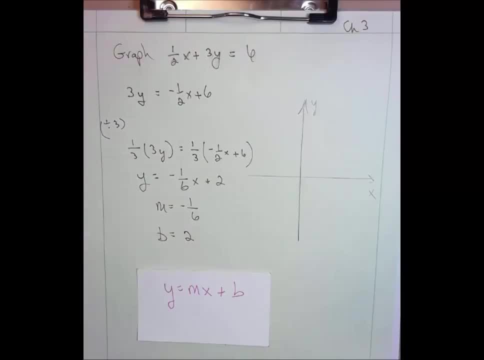 and a y-intercept of 2.. And so now I can place this line appropriately. It's very faint, but I'm going to consider every little tick mark on this graph paper to be half a unit. And so the y-intercept of 2, there's half 1, 1 and a half 2.. 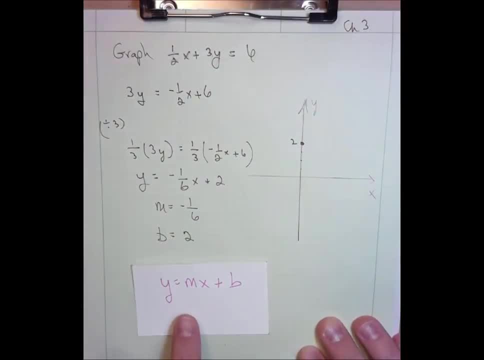 There's a y-coordinate of 2.. And then to count off a slope of negative 1 sixth, that means I'm going downhill and I'm going down by 1 for every 6. I move horizontally. So remember: rise over run.